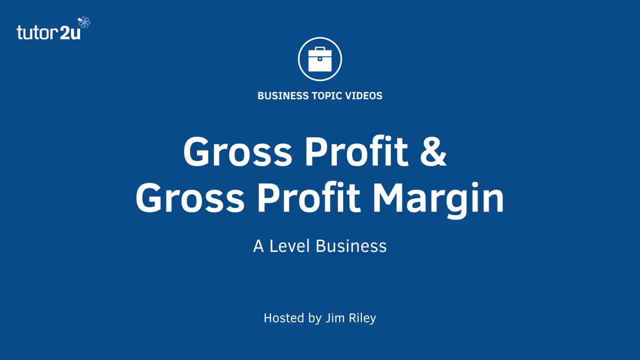 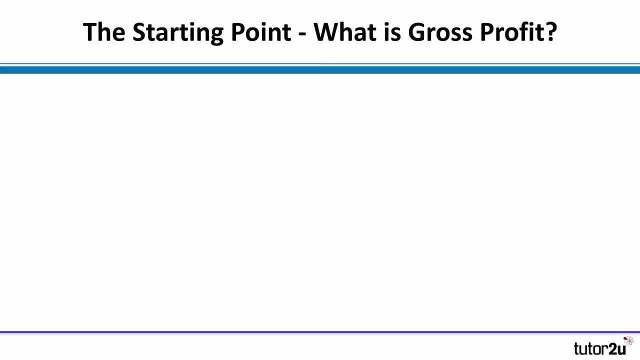 Hi there, Let's take a look at a really important measure of profit and profitability. It's the gross profit and the associated gross profit margin. The starting point for calculating gross profit margin is gross profit. So what is it? Well, it's the difference between the sales. 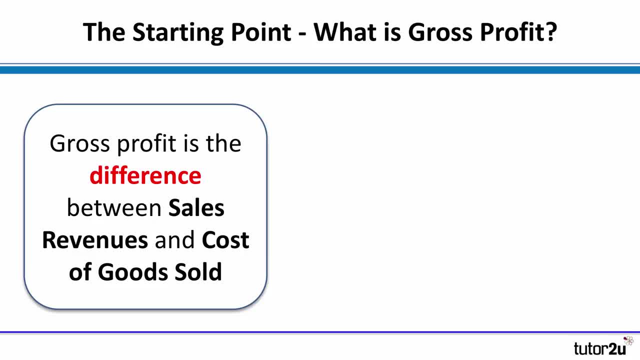 the revenues that we earn and the specific costs of those sales revenues, the so-called cost of goods sold. So it's not all the costs of the business, it's just the costs directly relating to those sales revenues. So, for example, if we had sales revenues of, say, 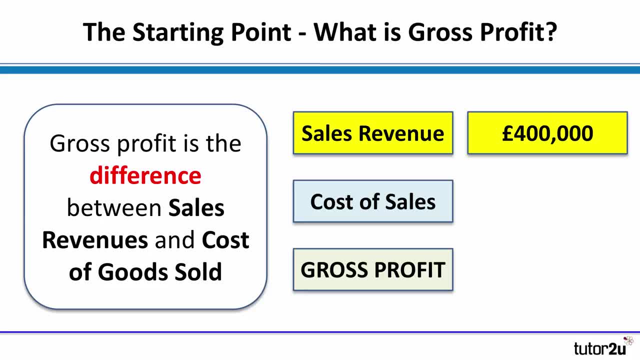 £400,000, and the cost of those sales was £150,000,, then the gross profit is simply the difference between sales revenue and cost of sales. So £400,000 less £150,000 gives us a gross profit of £150,000.. So the gross profit of those sales revenues is simply the difference. 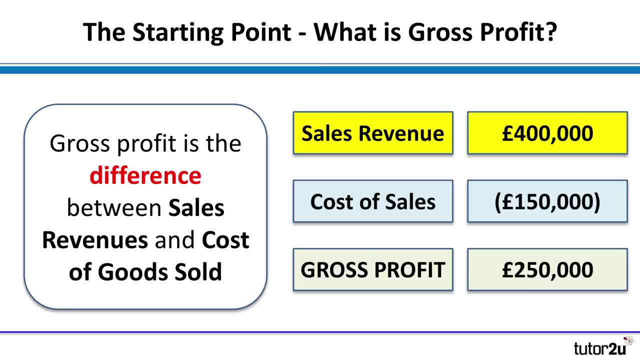 of £250,000.. That's not the total profit of the business, because we need to take off other costs such as overheads, but it's a really important measure of profitability. What's the gross profit margin then? Well, the gross profit margin is expressed as a percentage. 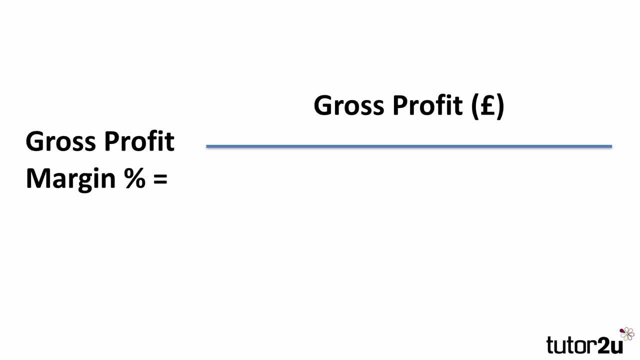 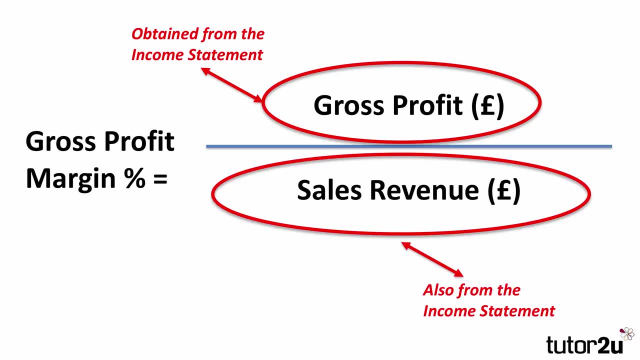 and the formula is the gross profit number divided by the sales revenue number, And we get both of those two pieces of data from the income statement: Sales revenue, the total value of sales, gross profit, which, as we've seen, is sales revenue less cost of sales, And we 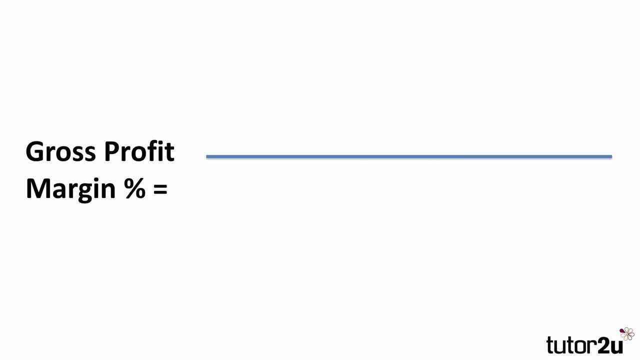 express the gross profit margin as a percentage. So, looking at that from our simple example at the start of this video, the gross profit divided by the sales revenue, the gross profit we worked out was £250,000 divided by the sales revenue of £400,000, always expressed as a percentage. So 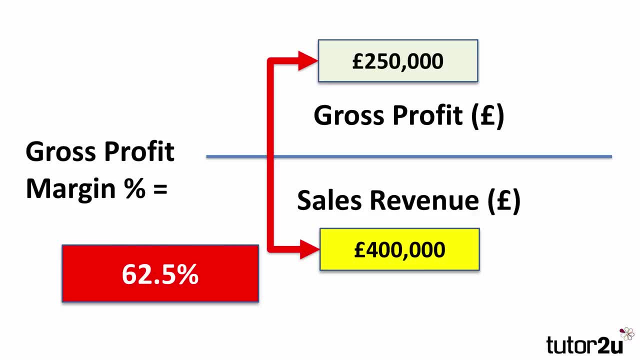 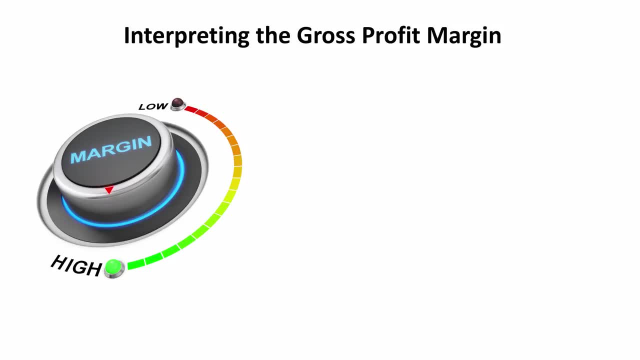 times by 100, that gives us a gross profit margin of £62,500.. Now, the gross profit margin is one of those margins that is really worth investigating and examining, particularly when we're comparing the performance of one business with another. So not only do we need to look out for changes from one year to another, 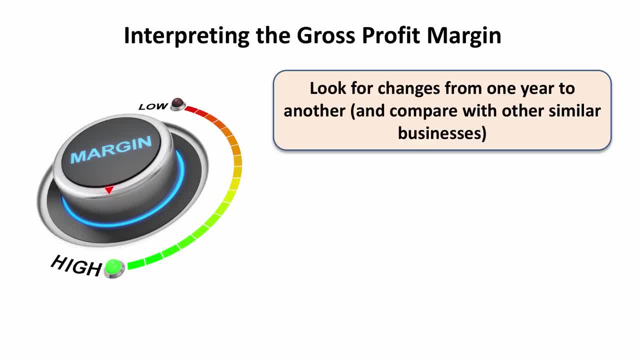 an increase or decrease in the margin, but also, how does the gross profit margin compare with competitors, Because in theory they should have similar gross profit margins. If the gross profit margin has fallen, there could be a number of reasons for this. It could be that the cost of good sales has gone up. Perhaps suppliers are charging us a higher.